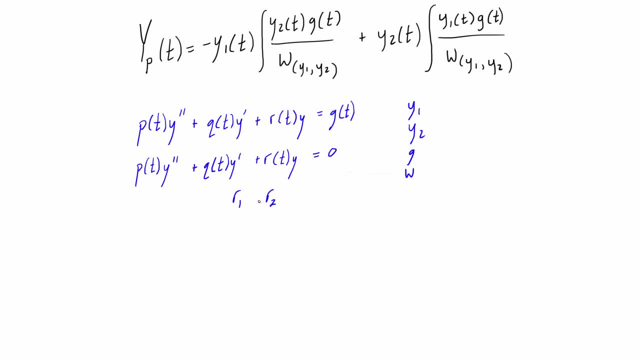 are real and distinct, or real and repeated or complex, you'll be able to write the general solution to the homogenous version. So let's say they were real and distinct, You would have yc of t. So yc of t is the complementary solution to the original differential equation, but it's also 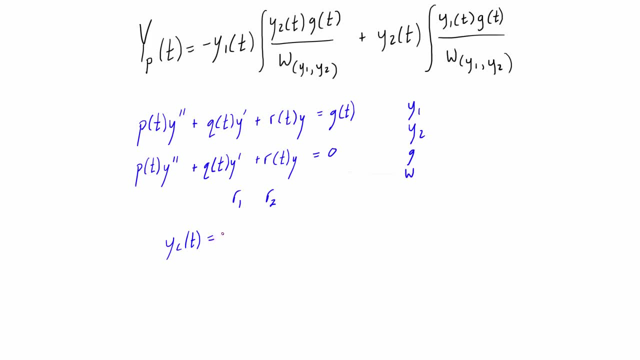 the general solution to the second-order differential equation. So you're going to homogenous version. And if these were real and distinct, the form would be basically just c1e to the rt, r1t plus c2e to the r2t. Now, if these were real and repeated or complex, the form would 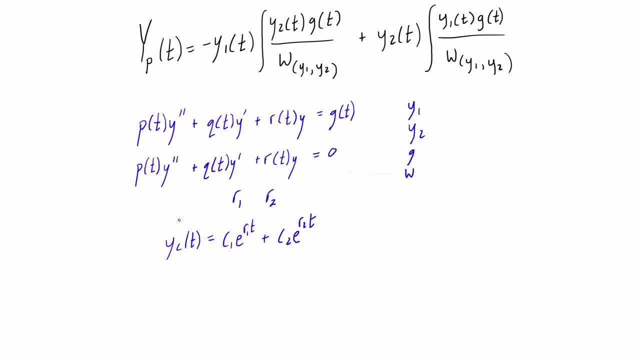 be a little bit different And we've gone over that in previous videos earlier in the course. But this actually has the form c1y1 plus c2t, So we can see here that we know what y1 is and then we also know what y2 is. So here we have. 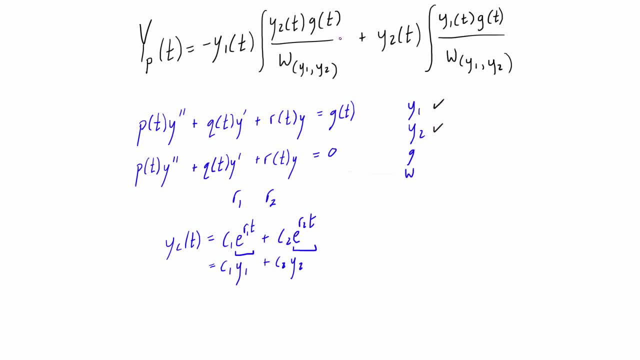 y1,, we have y2.. We have g of t because it's given to us in the problem, And then we can just lastly find the Vronskian. And if you remember, the Vronskian is just the determinant of this little. 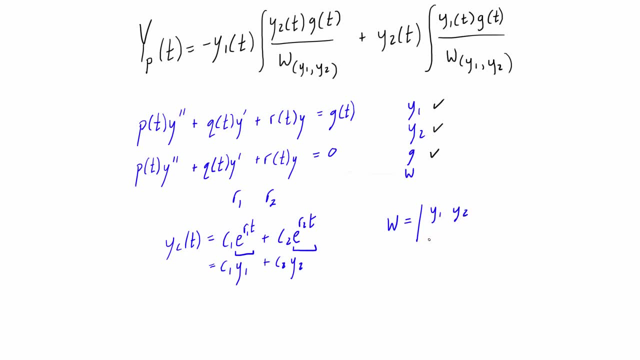 matrix here where we have y1, y2, and then y1 prime and y2 prime. So if we have y1 and y2, we can pretty easily find out what their derivatives are. We plug it into a little 2 by 2 matrix and we take the determinant. And now we also have something. 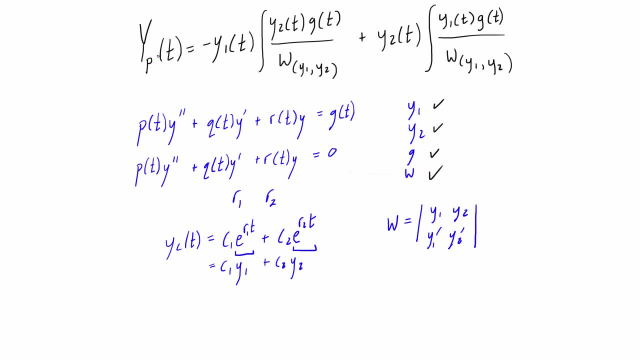 for w, And all we have to do is plug all of these into this expression and just crunch away and solve for the particular solution, yp of t. Now, this will work for a lot more cases than the undetermined coefficients method, which was the previous one that we were talking about. 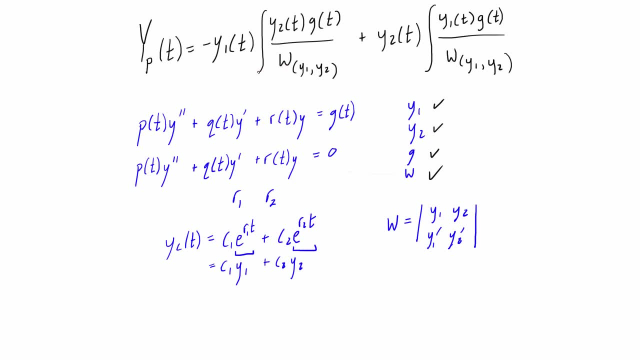 But I think what I'm going to do in the next video is I'm going to do a little bit more in the next couple of videos- is just solve the same examples that we were doing in undetermined coefficients, just so you can compare and see the differences in the two methods with the exact 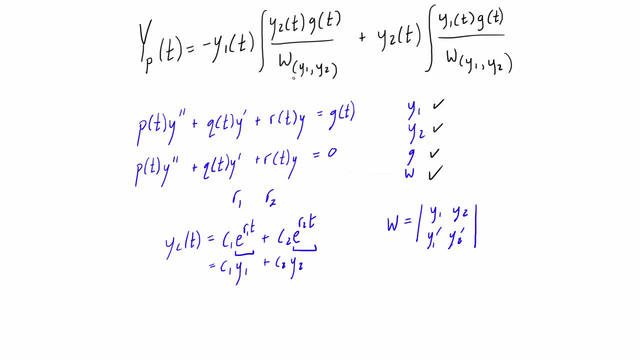 same problems. I think that's helpful. But just remember that this method, the variation of parameters, is applicable to a much wider set of possibilities that we can solve for the form of g, of t. But you'll see when I go over the next couple examples that sometimes just integrating here, just 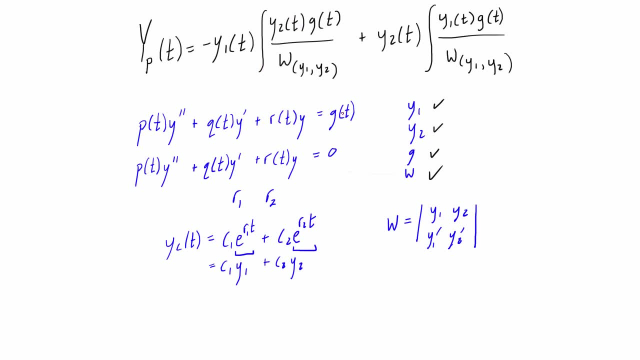 is like a beast, And if you're able to use another method, for example undetermined coefficients- sometimes with certain situations it's easier, but you're not always able to. So it's good to know how this works. and join me in the next couple of videos, And we're going to go over some examples and 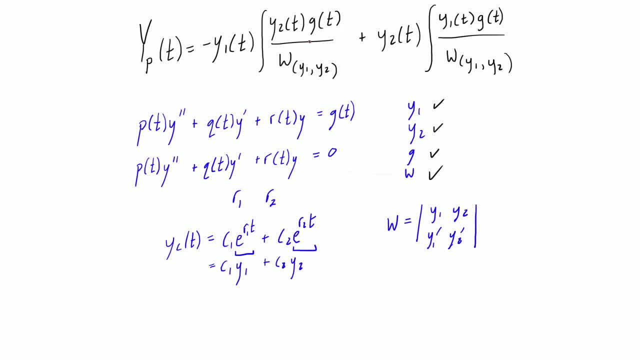 we're going to get pretty deep into integrating by parts which I know you all love. 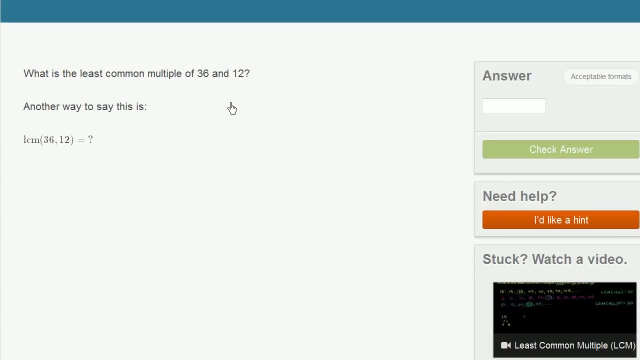 What is the least common multiple of 36 and 12?? So another way to say this is LCM, in parentheses: 36 and 12.. And this is literally saying what's the least common multiple of 36 and 12?? Well, this one might pop out at you. 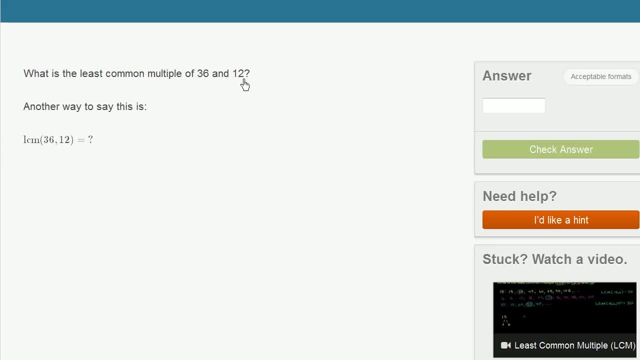 because 36 itself is a multiple of 12.. And 36 is also a multiple of 36.. It's 1 times 36.. So the smallest number, that is both a multiple of 36 and 12, because 36 is a multiple of 12, is: 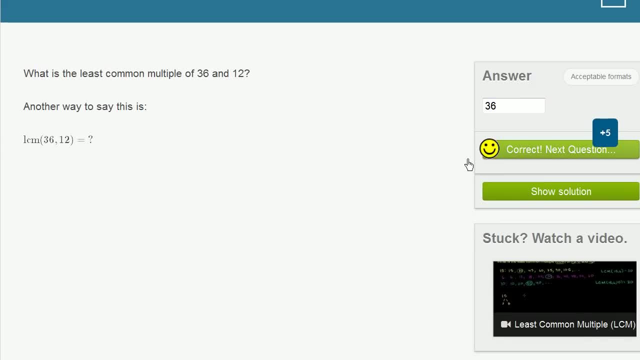 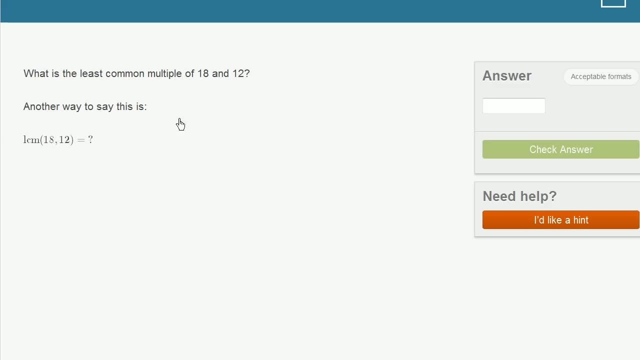 actually 36.. There we go. Let's do a couple more of these. That one was too easy. What is the least common multiple of 18 and 12?? And they just state this with a different notation: What's the least common multiple of 18 and 12? 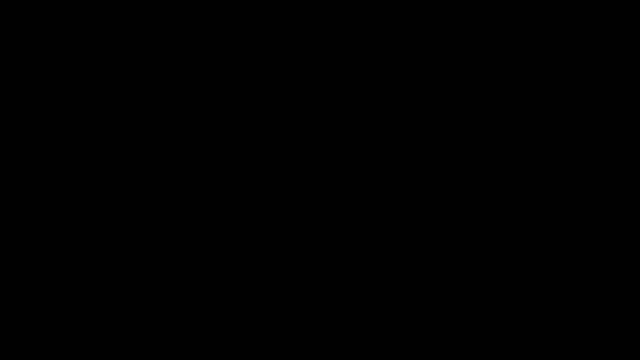 is equal to question mark. So let's think about this a little bit. So there's a couple of ways you can think about. So let's just write down our numbers that we care about. We care about 18 and we care about 12.. 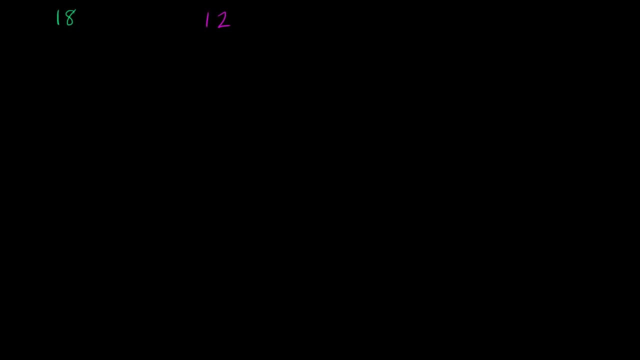 So there's two ways that we can approach this. One is the prime factorization approach. We can take the prime factorization of both of these numbers and then construct the smallest number whose prime factorization has all of the ingredients of both of these numbers. 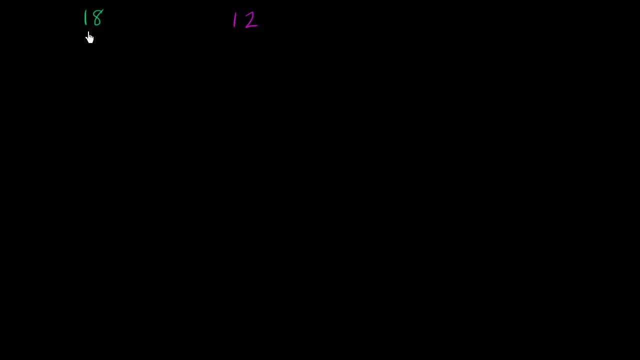 And that will be the least common multiple. So let's do that: 18 is 2 times 9,, which is the same thing as 2 times 3 times 3, or 18 is 2 times 9,, 9 is 3 times 3..